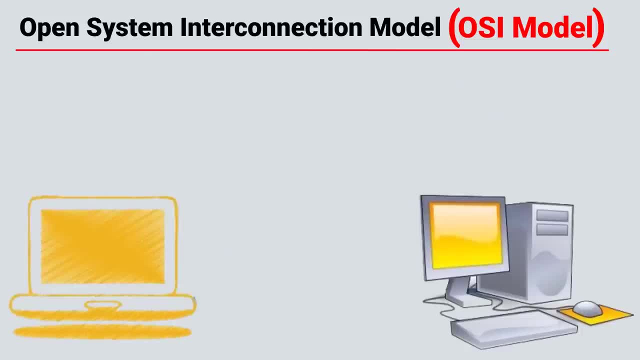 the globe. For example, there are two computers connected to each other via ethernet cable and RJ45 connector, sharing data with the help of network card. If one computer running on Macintosh operating system and other one having Windows 10, then how these two computers with different operating system are going to communicate to each other? 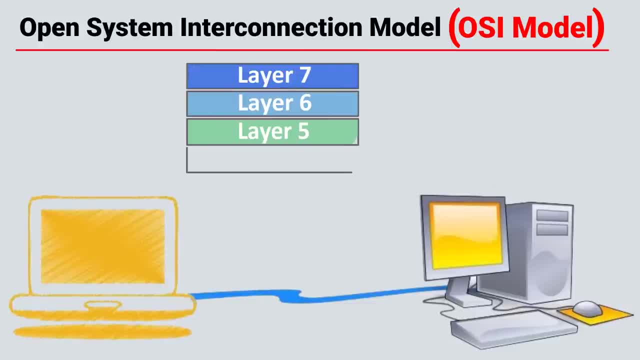 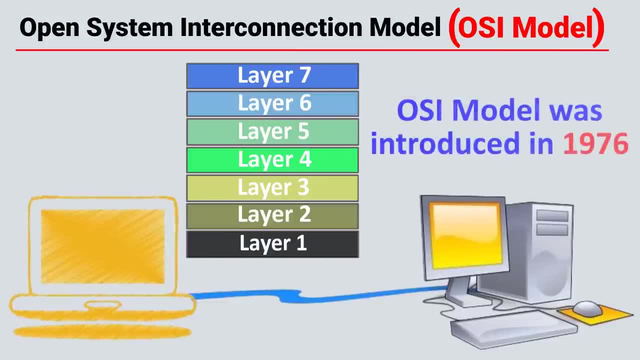 To solve this issue and for successful communication between two computers or networks, open system interconnection model, or OSI model, was introduced in 1976.. The OSI model developed by international organization for standardization, or simply called ISO. The purpose of OSI reference model is to 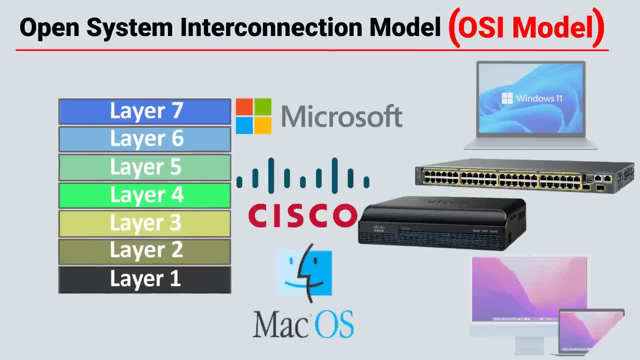 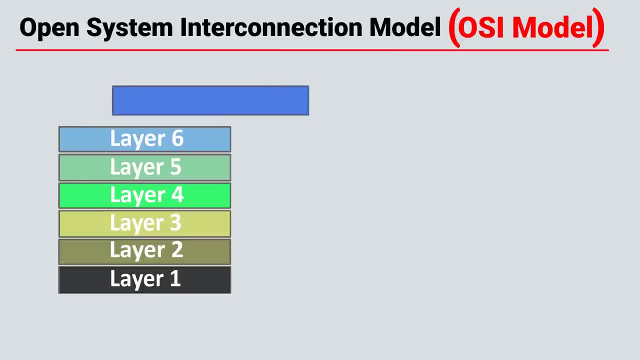 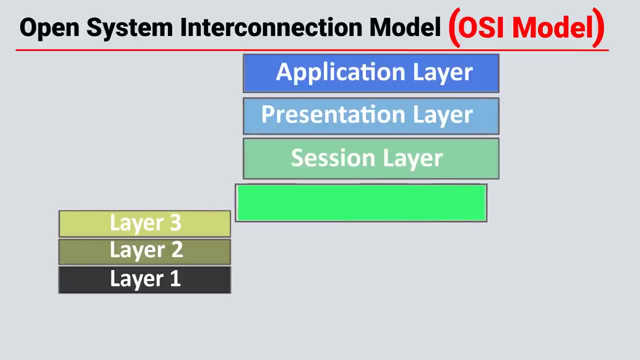 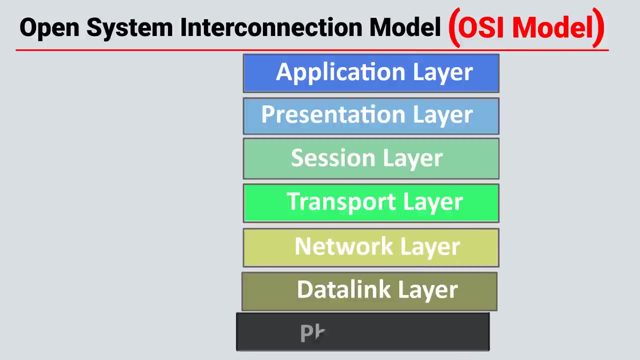 guide technology vendors and developers so their hardware and software can inter-operate and define the common framework. There are seven layers in OSI model. from top there is application layer, then presentation layer, session layer, transport layer, network layer and physical layer. If you feel difficult to remember OSI model layers name and their sequence, 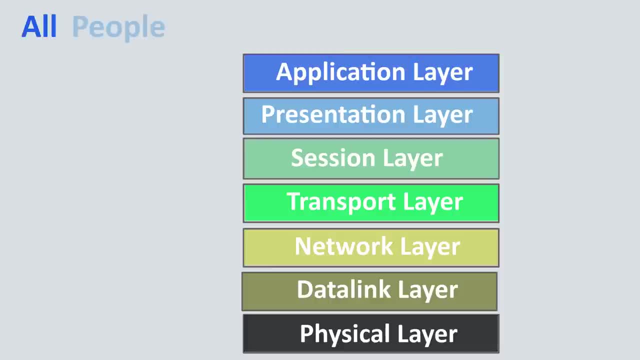 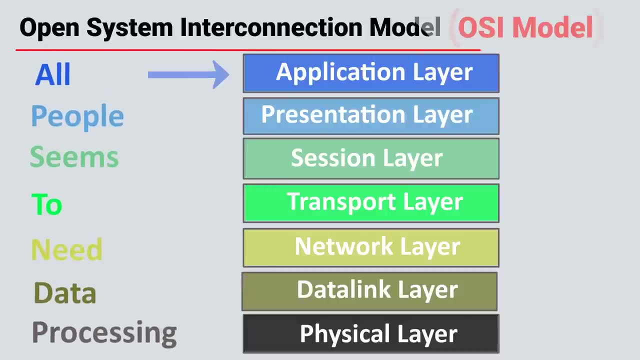 then try to remember this phrase: all people seems to need data processing, Start from top to bottom. A from all means application, layer P from people means presentation. layer S to session. layer T to transport. layer N to network. layer D to datalink layer. 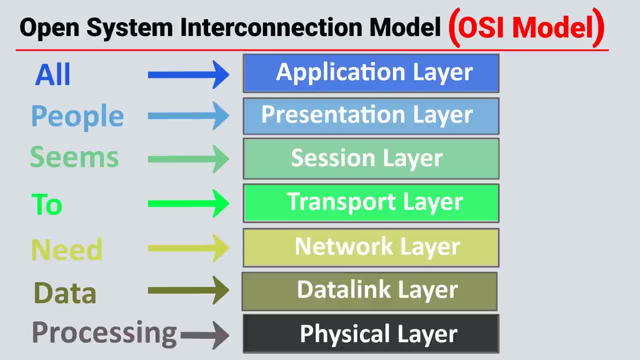 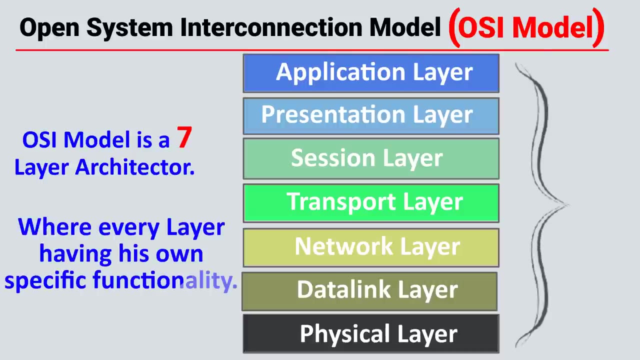 and P for physical layer. So to remember this single phrase, you will always remember OSI model layers name and their sequence. It's very famous phase and I hope so many of you already know it. OSI model is a seven layer architecture where every layer having his own specific functionality. 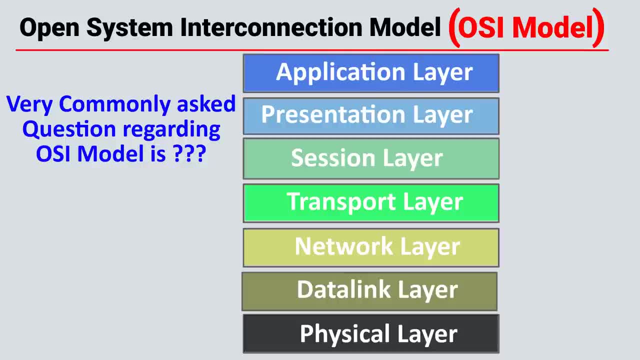 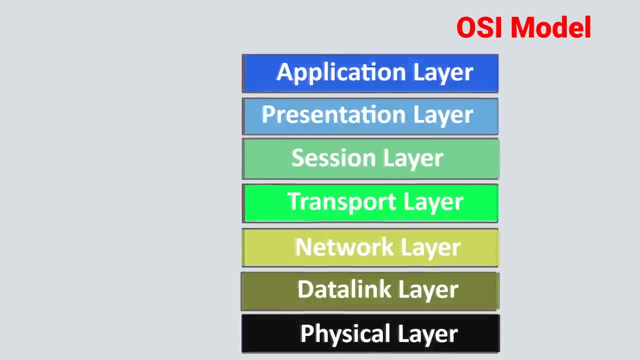 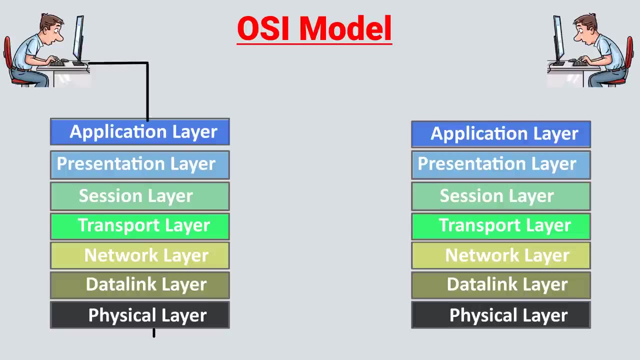 Very commonly asked question regarding OSI model is: which layer is first layer of OSI model, On top of all application layer or bottom one? To answer this question, always remember it's depend on your position, means you are on sender side or on receiver side. See, if you are on sender side, then top layer of OSI model or application layer. 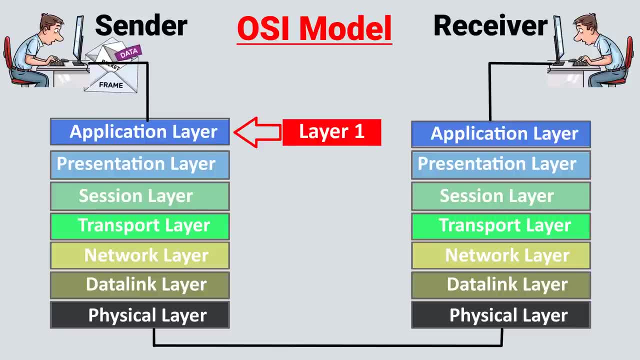 is your layer one because, as a sender, you will interact or come in touch with application layer. first Because, as a sender, when you work on any application like Google Chrome, Facebook or Yahoo, they will use application layer protocols like HTTP, HTTPS or SNMP to send the data. But if you are on receiver side, then the first. 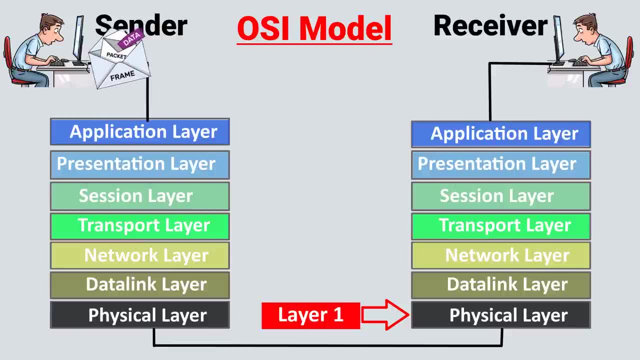 OSI layer is physical layer because as a receiver you receive data and first layer who interact with data is physical layer. So your layer one is depend on your location: you are on sender side or on receiver side. All the seven layers work together in collaboratively to transfer data from. 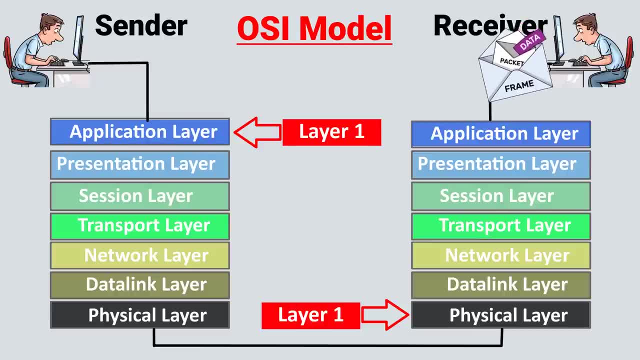 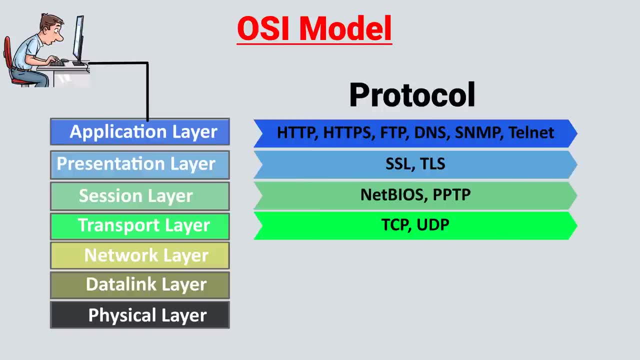 one computer to another computer in the network or across the globe. Also note each layer having his own protocols to perform his job. That will be explained and discussed into another video with details. The top three layers: application layer, presentation layer and session layer. 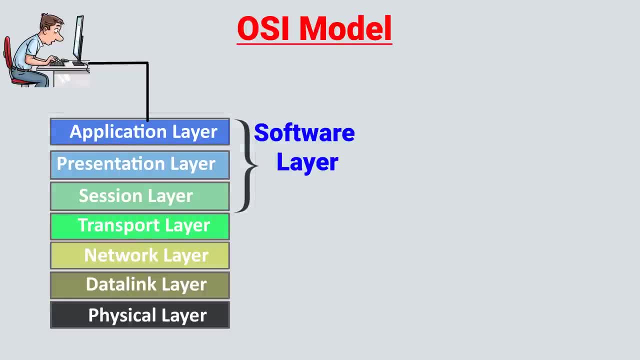 are also called software layer because application software like Google Chrome, Firefox, Facebook, Gmail and file sharing application like Dropbox protocols are exist and work in application layer. The bottom three layers- network layer, data link layer and physical layer- are called hardware layer because network hardware like router, switches, hub, UTP cable and RG4 network are 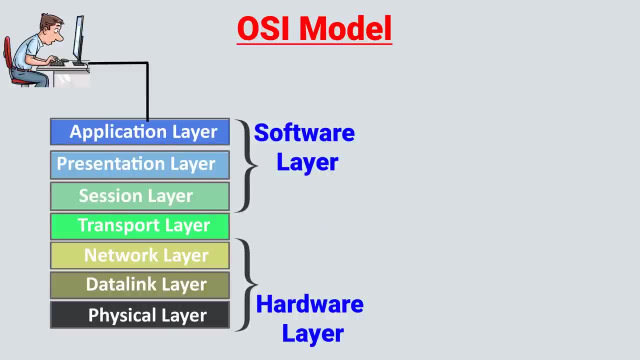 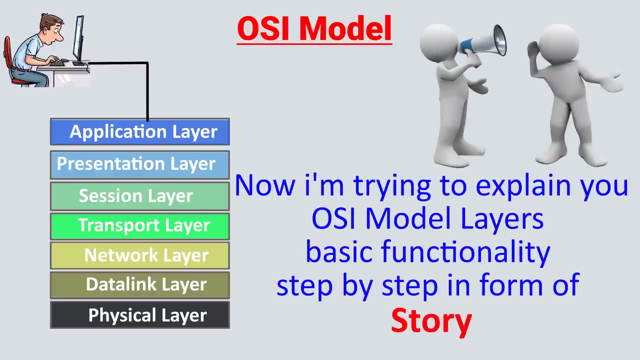 used in these layers. The middle one, or transport layer, is called backbone of OSI model or heart of OSI model, because it make a connection between top layers, or software layers, and hardwares, or bottom layers. Now I am trying to explain you OSI model layers basic functionality step by step, in form of: 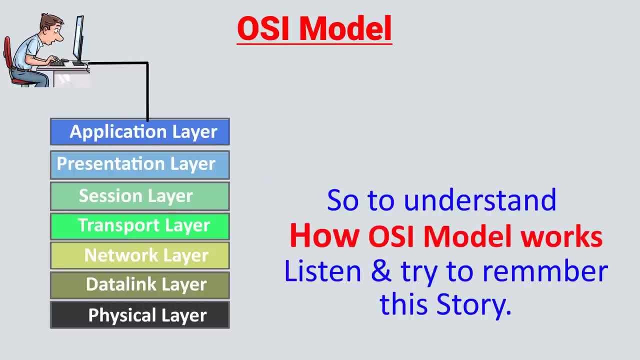 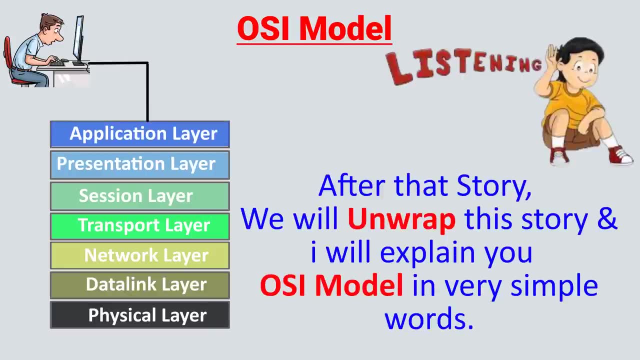 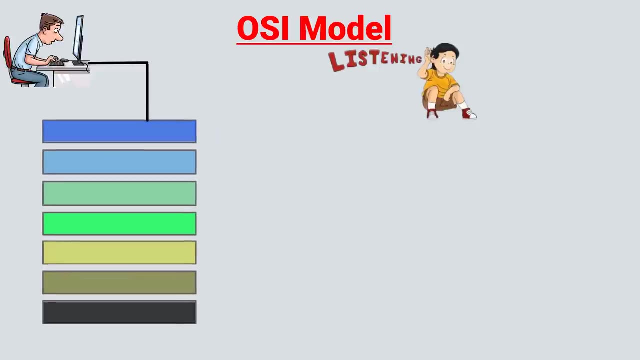 story. So to understand how OSI model work, Listen and try to remember this story. After that story, we will unwrap this story and I will explain you OSI model in very simple words. So let's start it Just assume there is one company in Qatar and they have seven employees. 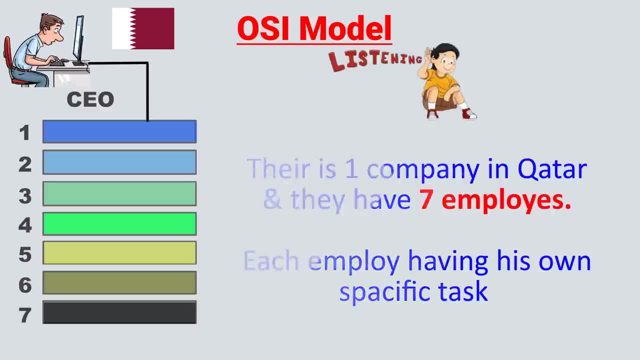 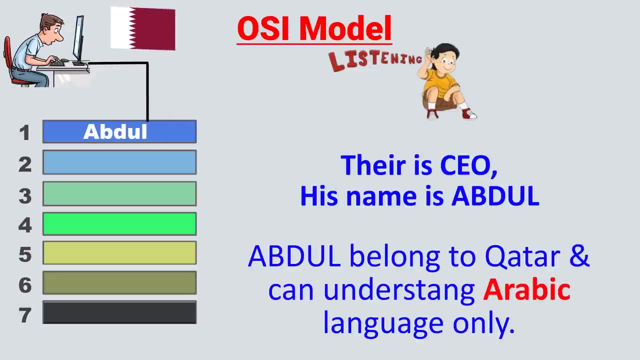 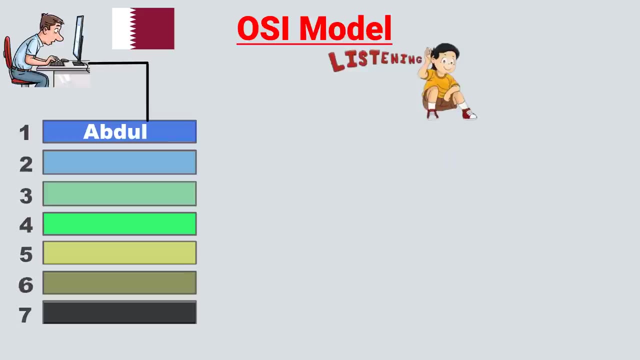 Each employee having his own specific task. On the top there is CEO of the company and his name is Abdul. Abdul belongs to Qatar and can speak and understand Arabic language only. There are another six employees who working in Abdul company. Their names: 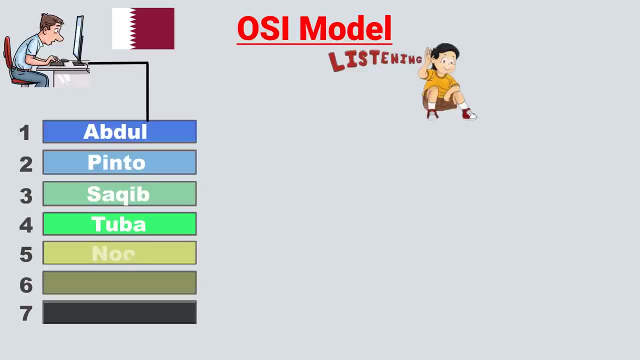 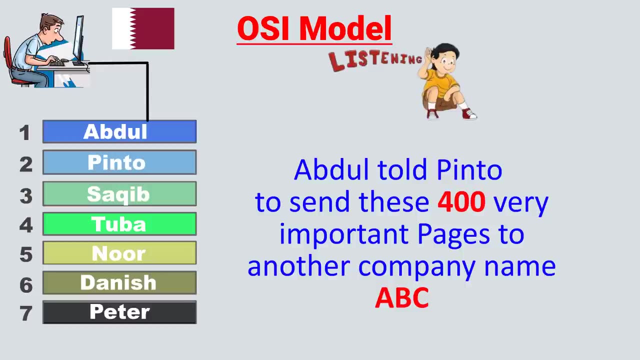 are Pintu, Saqib, Tuba, Noor, Danish and Peter. The CEO of the company, Abdul told Pintu to send this 400 very important pages to another company named ABC and make sure it delivered. Pintu say okay, boss, and take 400 pages from Abdul and 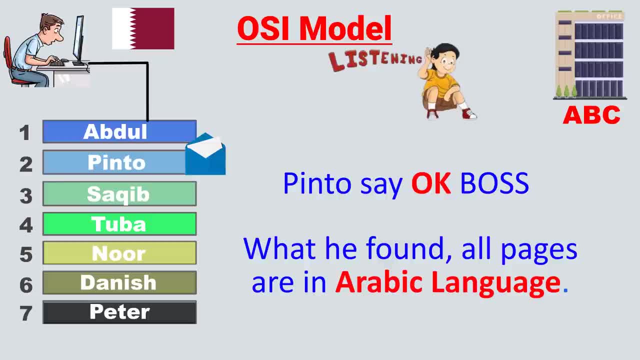 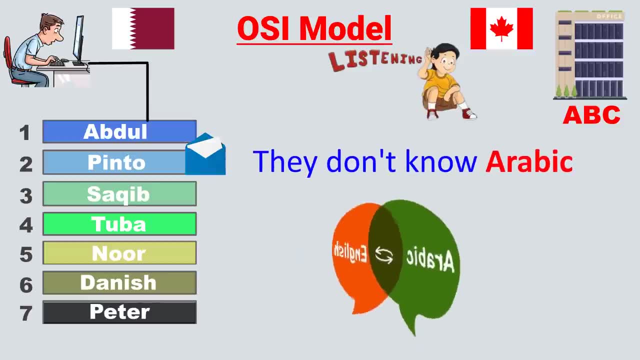 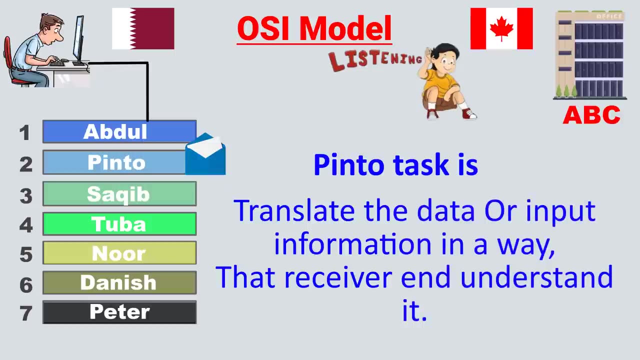 what he found? all pages are in Arabic language, but the ABC company in Canada? they don't know Arabic. So what Pintu did? he convert these 400 pages into English first. So Pintu task is translate the data or input information in a way that 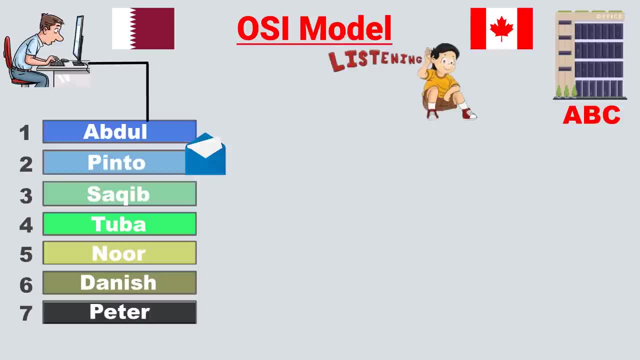 receiver and understand it. So, after converting Pintu, hand over this 400 pages data to Saqib and inform Saqib. these 400 pages are very important and will be sent now to company name ABC. When Saqib receive and check it will go. 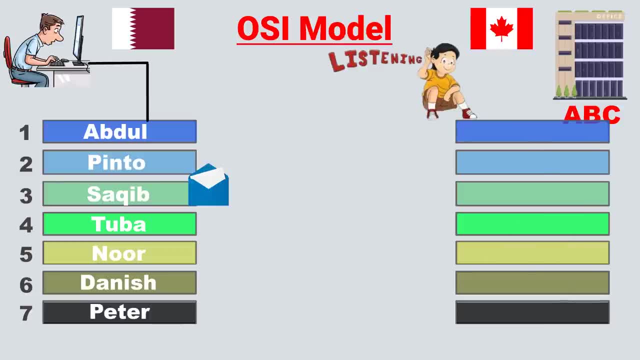 to company name ABC in Canada. So Saqib contact to ABC company first on his equivalent position person and ask: is your company open now? They replied yes. Then Saqib inform there is one document coming to your company from us and when you receive it, please confirm us or send acknowledgement that you receive our. 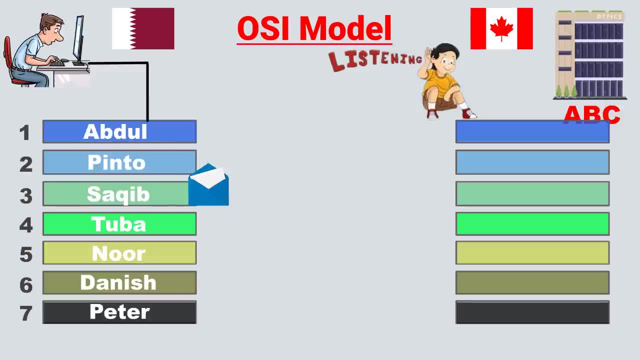 document. They say okay, And they both agreed to establish a connection between sender and receiver until they not receive the data. So, Saqib, create end-to-end connection between sender and receiver and then hand over these 400 pages to Tuba. Tuba found. 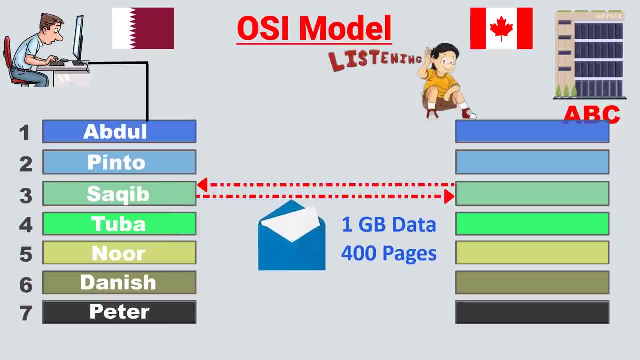 there is big data file with very important and confidential 400 pages. So what Tuba did? she divide these 400 pages into four sets of hundred pages or segments, and mark these segments as segment one, segment two, segment three and segment four, Because big file take more time to send from one place. 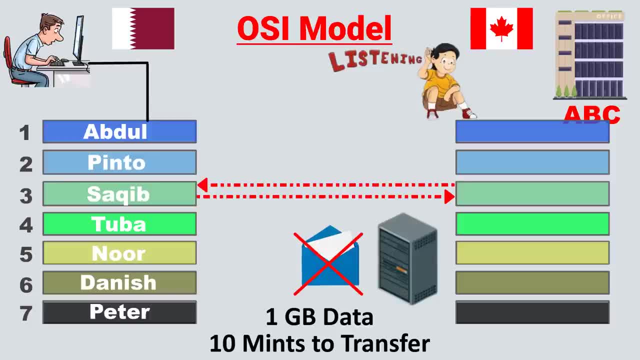 to another. also, if they lose that file, they lost all data at once, But in other hand Tuba divide them into small bundle or segment and if one segment lost, other data will be safe in other segments After data segmentation. Tuba sent this four bundle to Noor. Noor receive four bundles from Tuba and 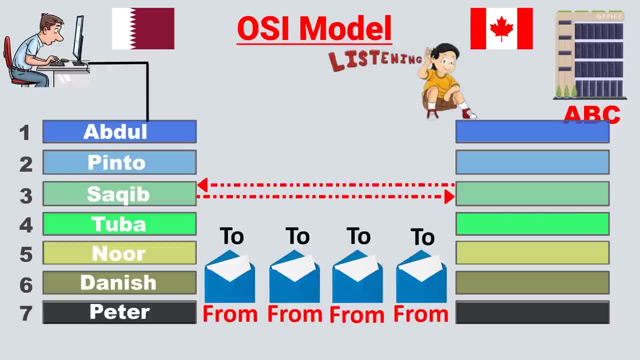 she write to and from address on each bundle or packet. On to, Noor mention receiver or ABC company address in Canada and on from side she mention his company address in Qatar. Also, Noor inform delivery man: these are very important papers and CEO want urgent to deliver, So don't send via normal post. 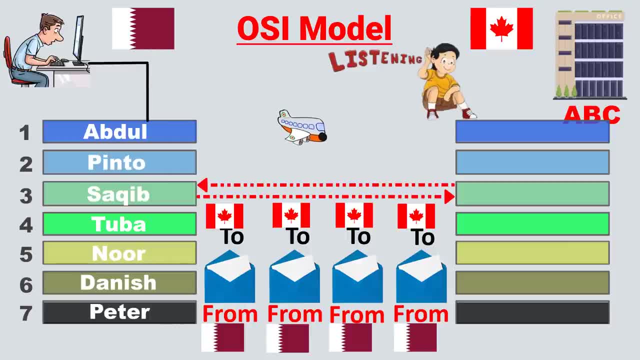 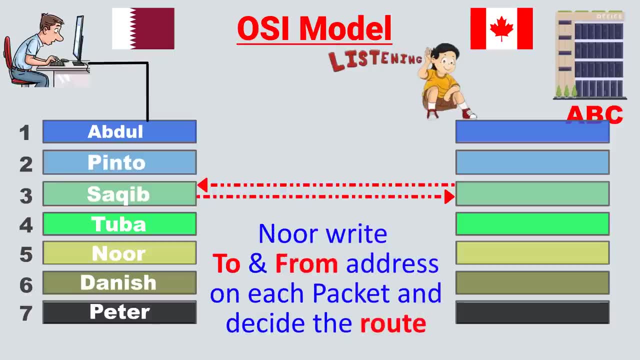 Noor instruct to take a flight from Qatar to Canada and deliver by yourself. So what, basically, Noor did? she write to and from address on each packet and decide the route. And after that, Noor sent these packets to Danish. Danish check each envelope and found: okay, Documents are. 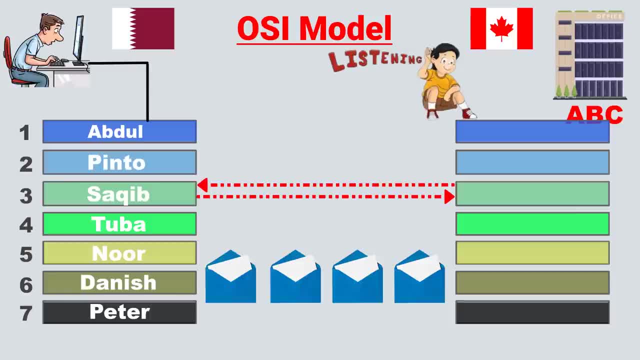 also inside on each envelope and sender and receiver address also mention on each envelope. but all envelopes are open. Anyone can see and read this documents. Then what Danish did? he close all envelopes and put seal on it to protect the envelopes. So if anyone try to open those envelopes, 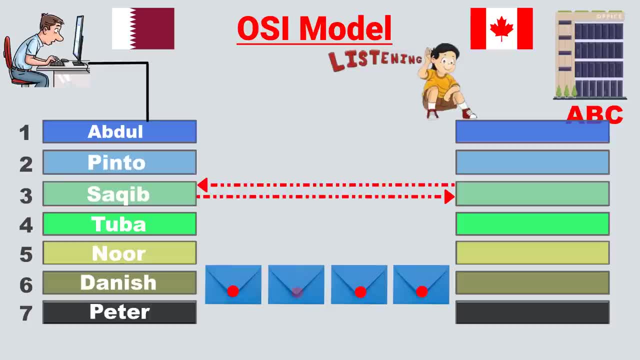 Receiver know that someone tried to tamper the documents After this. Danish handover this envelope to Peter and told Peter to send this envelope to ABC company in Canada. Peter go to ABC company in Canada and handover this envelope to receptionist in ABC company. 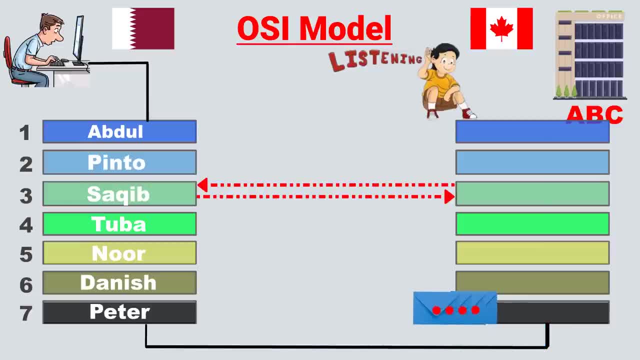 Receptionist receive the delivery and send to next department. That department check all four envelopes are closed and sealed So no one tamper original documents. Then he open the envelopes and send document to next department. Next department check the to and from addresses and confirm this is his company address and 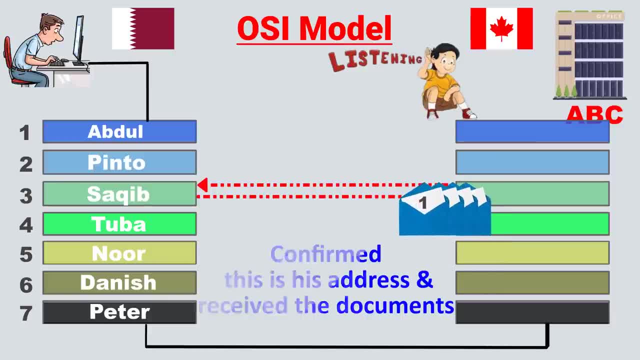 receive the document and send to next department. When next department receive that all four envelopes and they check there are envelope 1, envelope 2, envelope 3 and envelope 4.. Basically these are one document but in four different envelopes. What he did 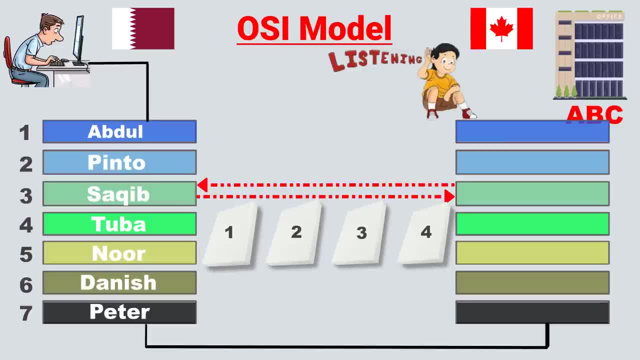 He open all four envelopes and put 100 pages from envelope 2 to under envelope 1 pages and envelope 3 pages under envelope 2 pages and envelope 4 pages under envelope 3 and make them as one bundle again of 400 pages and send to next department. 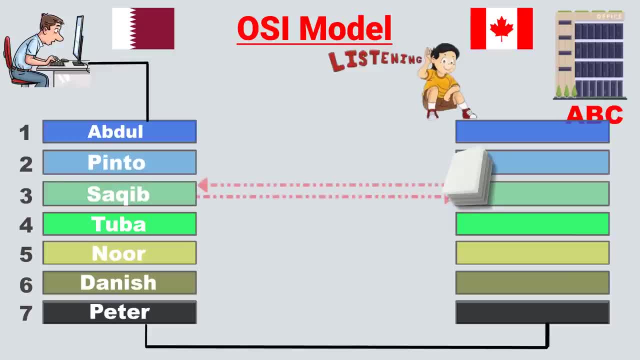 Next department. already in touch with sender and after getting 400 pages from lower level, he confirm to sender that they receive their documents. After confirmation, they discredit the connection and send this 400 pages to upper level. After acknowledgement or confirmation, the sender responsibility finished and after that, 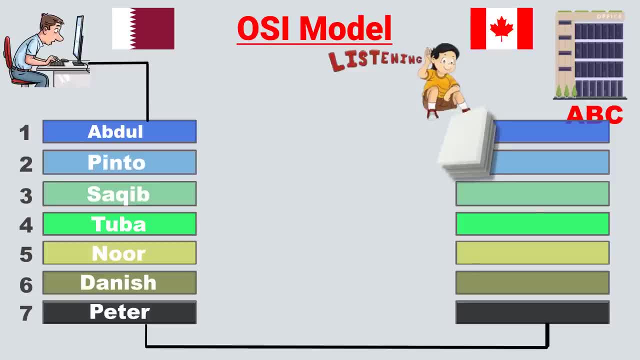 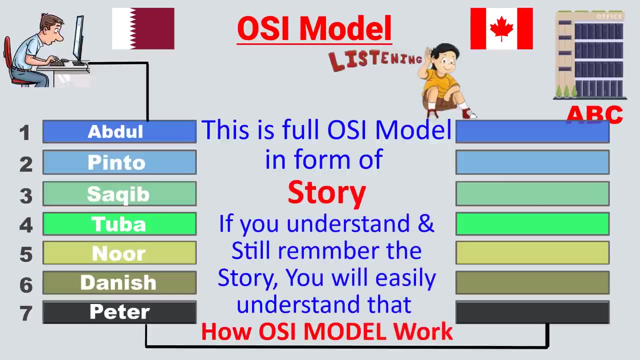 receiver, hire management. take a look on that document or no, this is not his problem. So what sender did? They all did their job, that is, deliver data from sender to receiver. This is full OSI model in story. If you understand and still remember the story, you will easily understand that how OSI model 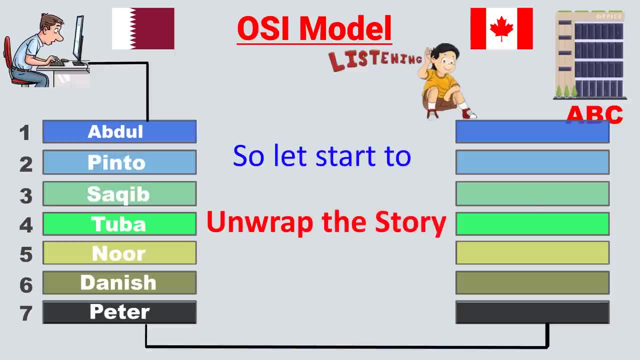 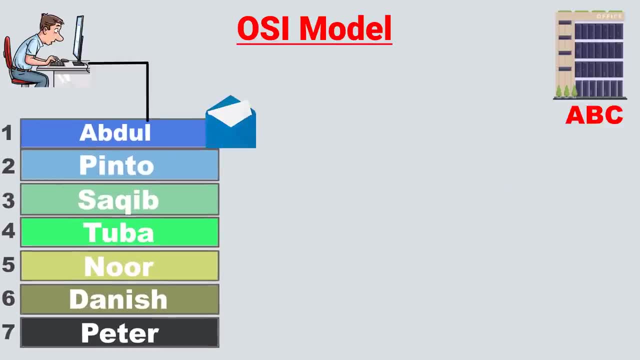 work. So let's start to unwrap the story. So first there is Abdul in the story. As per story, Abdul gave 400 pages to Pintu to send other company. Abdul means application layer as per OSI model, and that 400 pages mean any data that user. 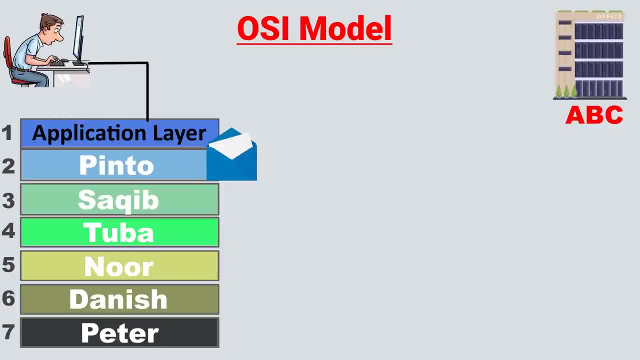 generate or create on application layer. So let's start. And application layer task is to provide interface to user. All applications and software we use in daily life, like Google Chrome, Firefox, Gmail, Yahoo or any file sharing application like Dropbox, that all work with the help of application. 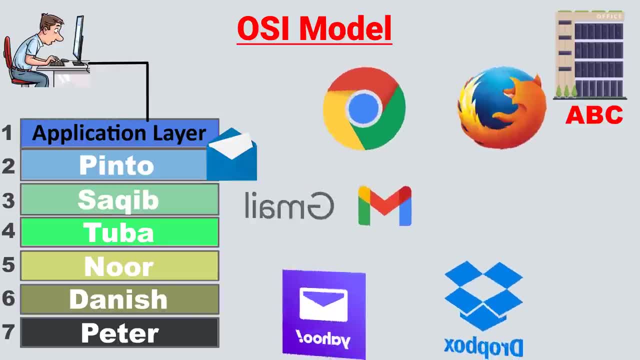 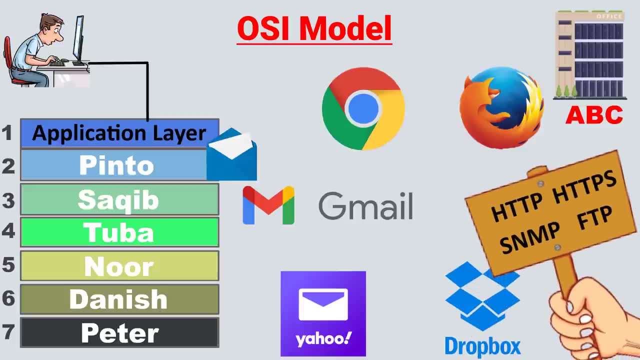 layer protocols- User basically work on applications, but it include application layer protocols that need to make this application to work correctly in the application. So let's start. Different type of application use different protocols, like if you browse something on Google Chrome or Firefox. they use HTTP or HTTPS protocol for web browsing. 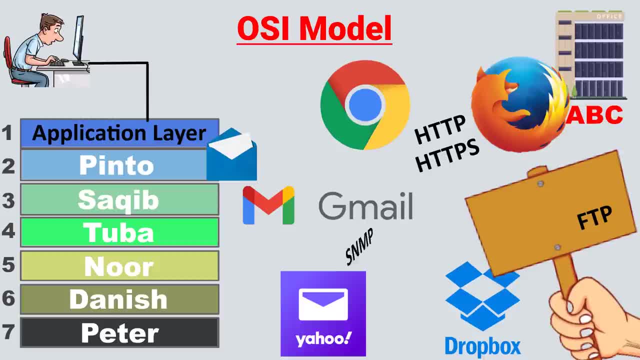 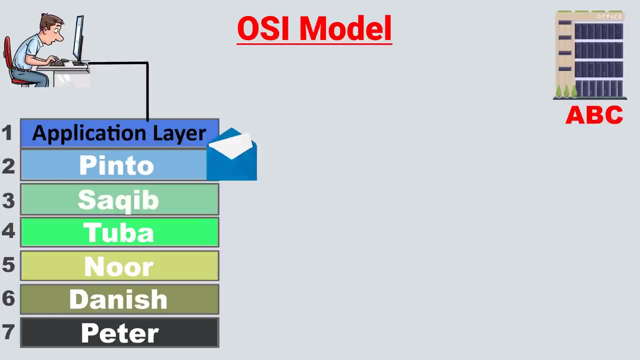 For email like Gmail or Yahoo, application layer use SNMP protocol. or if you transfer any file by using any file sharing website like Dropbox, that time application layer use FTP protocol To make this application to work correctly. So, as per story, Abdul give 400 pages to Pintu and what Pintu did? Pintu translate that pages. 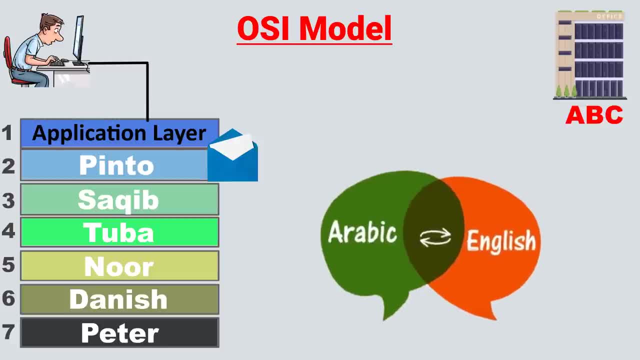 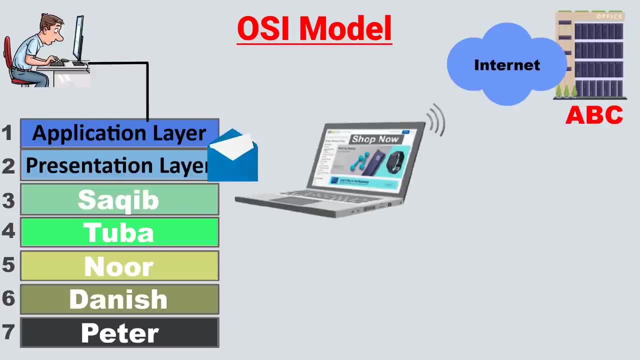 from Arabic to English because Pintu know other company don't know Arabic. Pintu means presentation layer as per OSI model. Basic function of presentation layer is convert application layer data into machine understandable binary format 1 and 0s. Also note presentation layer performing 3 functions: first, data translation. number 2: encryption. 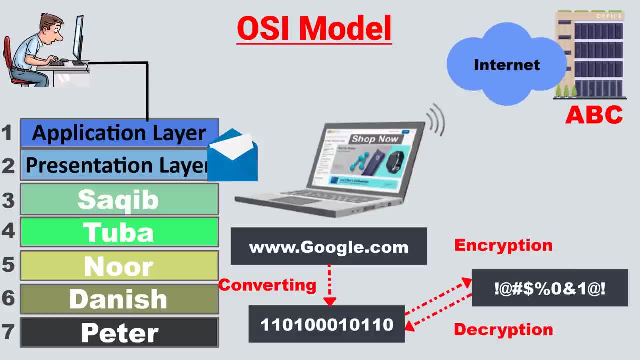 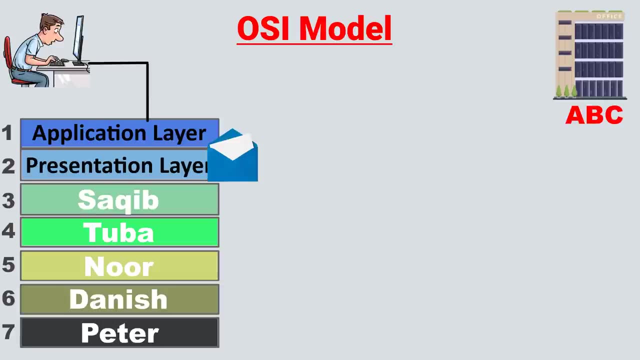 and number 3, decryption of data. So actually presentation layer function is data translation, data encryption on sender side and data decryption on receiver end. I explain you in simple words what presentation layer actually doing. You saw many time. there is audio file in your PC. 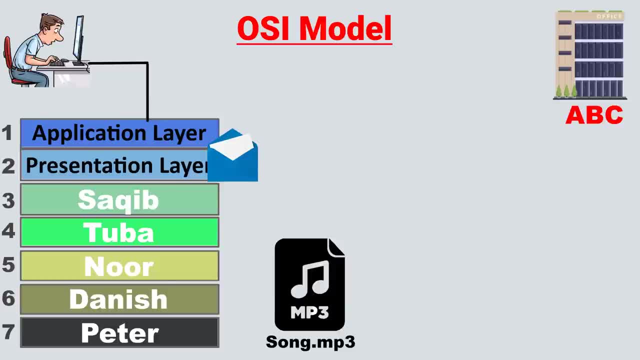 For example name songmp3 or something like that. You can also note presentation layer performing 3 functions: first, data translation. number 2, encryption. and number 3, decryption of data If you double click on document like filedocx or filepdf. If you double click on songmp3 file where it will be open. 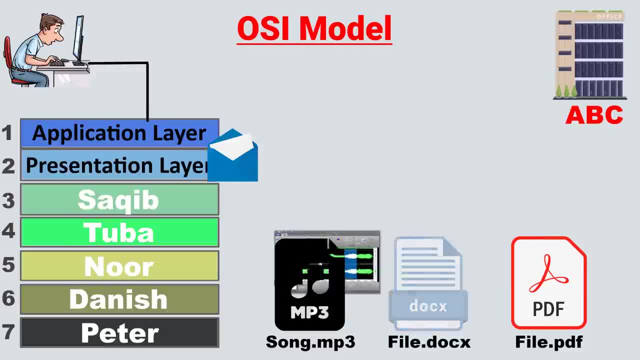 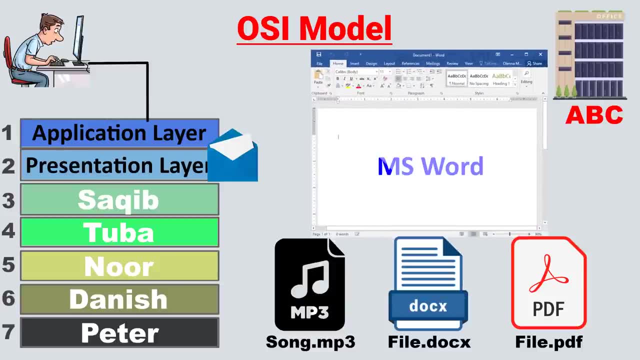 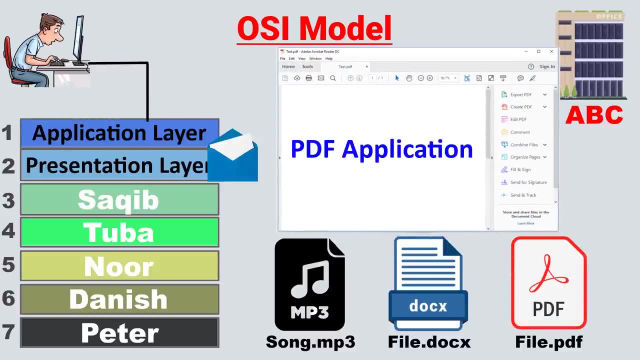 You will see it will open in mp3 player. or if you double click on filedocx, you will see it will open on different application like Microsoft, word or same. if you double click on filepdf, it will open in pdf application. Who telling this? 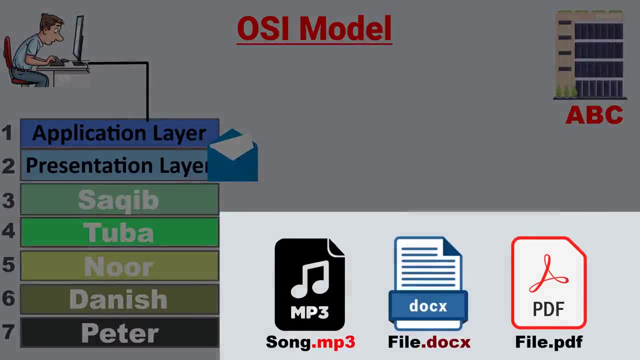 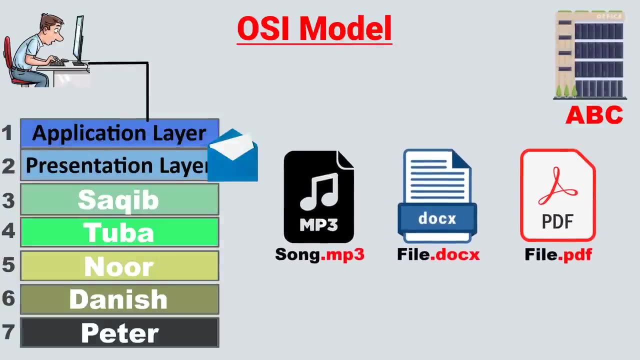 Where to open this file, That mp3 or tocx or pdf extension telling to computer. So that extension tell PC which application open this file. These extensions basically is the translation of application layer input. So presentation layer work is how to present data in form of mp3, tocx or pdf. 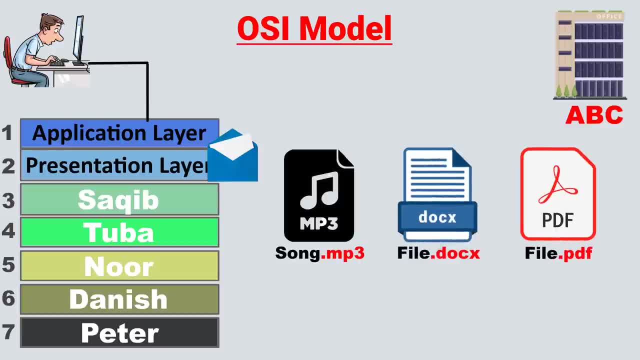 That's why in storypindu translate 400.. That's why in storypindu translate 400.. pages from Arabic to English because presentation layer task is present the data After: in storypindu send 400 pages data to sakip and sakip contact to receiver end and. 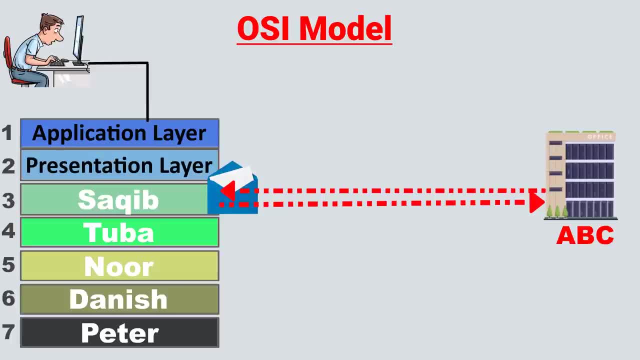 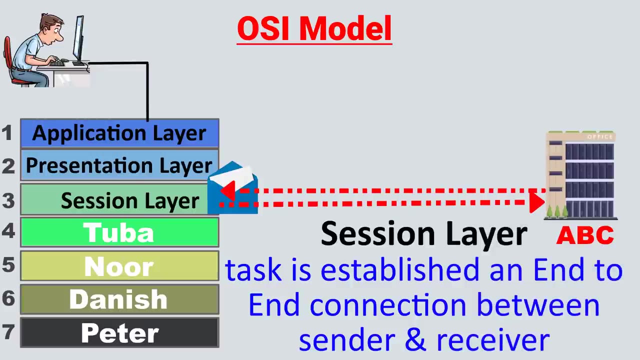 check their availability and establish connection. After establish connection, sakip inform them we are going to sending data and when you receive let us know. So sakip mean session layer in OSI model And session layer task is establish an end to end connection between sender and receiver. 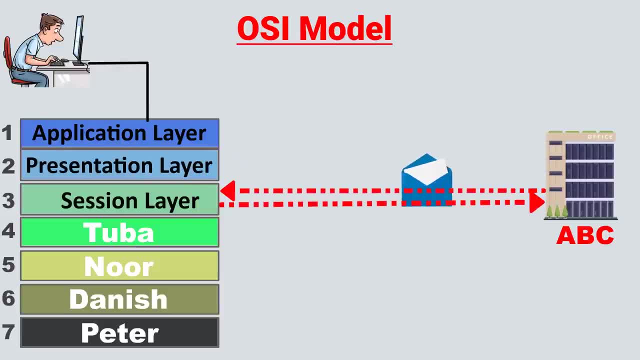 Both session layer keep connected until all data not received to other party. and if some data lost, sender get message from receiver end that data lost or unsuccessful. And if receiver end receive all data, then session layer get reply that data sent successfully. That's why session layer also called end to end layer. 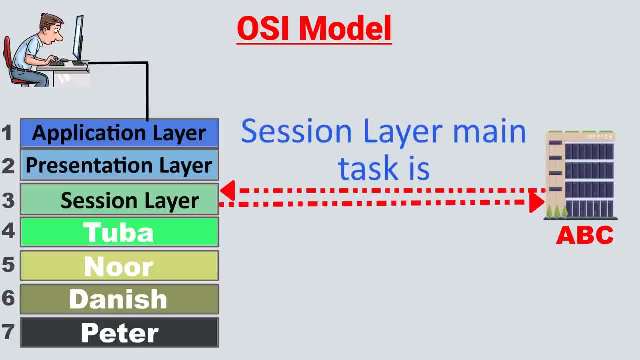 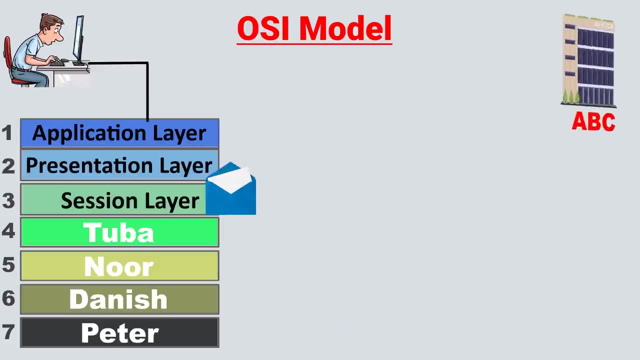 So session layer is also called end to end layer. That's why session layer also called end to end layer. So session layer main task is to ensure that all data received to other party without loss. Back to story: sakip, send this data to tuba. 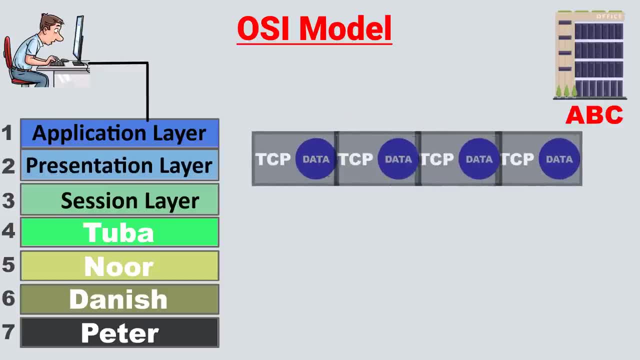 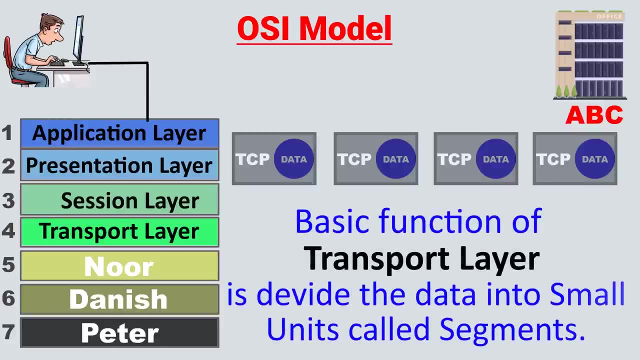 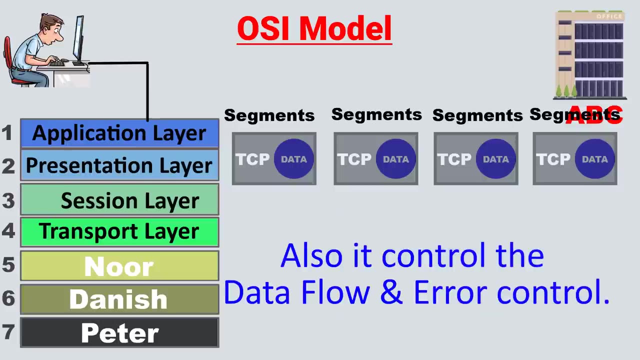 What tuba did tuba divide 400 pages into 100 pages in small units. Tuba stand for transport layer, as per OSI model, and the basic function of transport layer is divide the data into small units called segments. Also, it control the data flow. 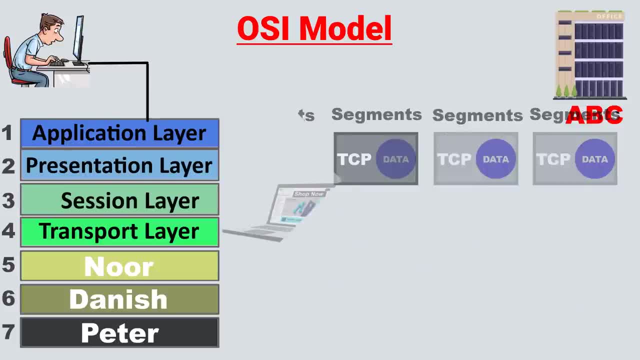 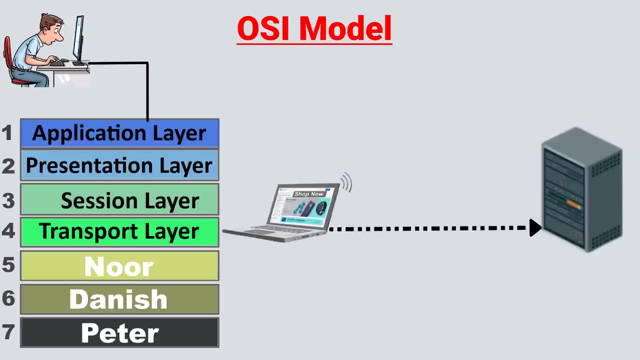 And error control In data flow control: transport layer control the amount of data being transmitted. For example, a laptop connected to a youtube server and suppose youtube server can send data at 100 mbps speed, but my laptop can process data maximum at 10 mbps speed. 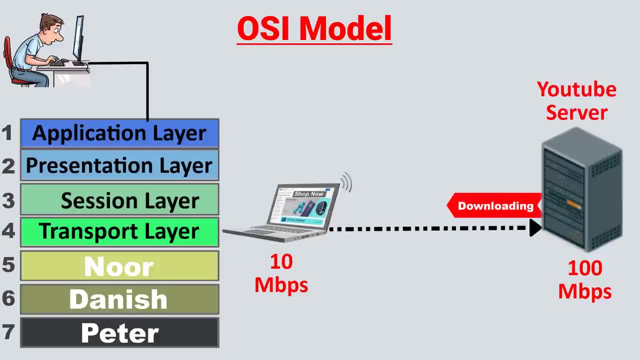 In that case, when I am downloading file from youtube server and server start sending data at 75 mbps speed, Which is greater than the data rate that my laptop can process. So by using transport layer, my laptop send request to server to slow down data transmission. 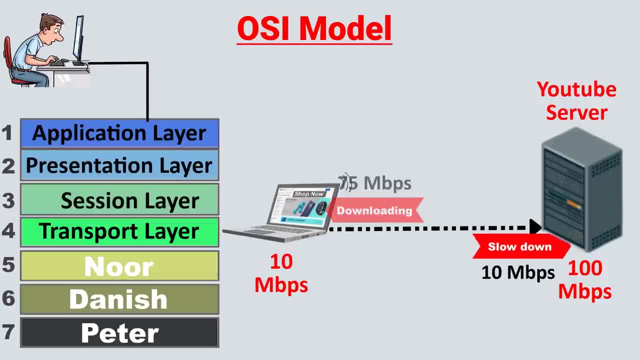 rate upto 10 mbps. That can maximum handle by my laptop and no data get lost. Same in reverse case: if server is sending data at 5 mbps, my laptop tell server to increase the data transmission rate at 10 mbps to maintain system performance. 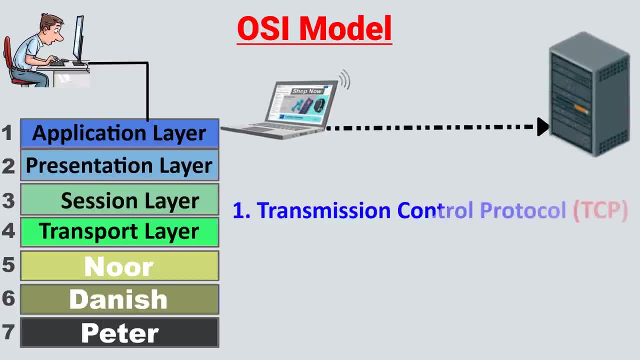 Also, there is two more things to consider. There is two type of protocol in transport layer: Transmission control protocol, or TCP, and user datagram protocol, or UDP. To get acknowledgement from receiver after receiving data or need to send any data segment again if data lost between transmission, we use TCP protocol. 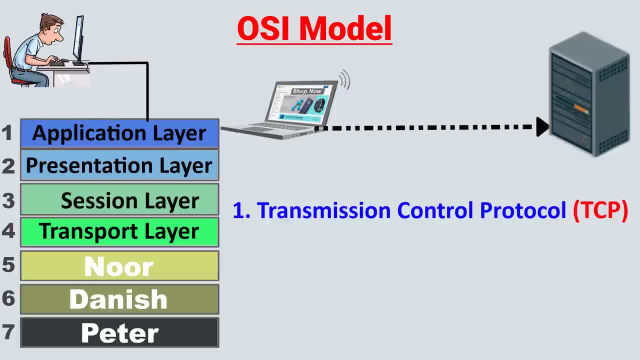 Its also called connection oriented transmission, TCP. send data at low speed and retransmit it again, also If some data lost. But if you want to send data on fast speed without establish session and don't care it it received on other side or no, 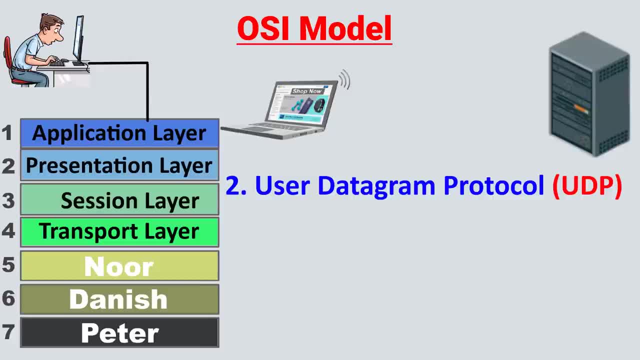 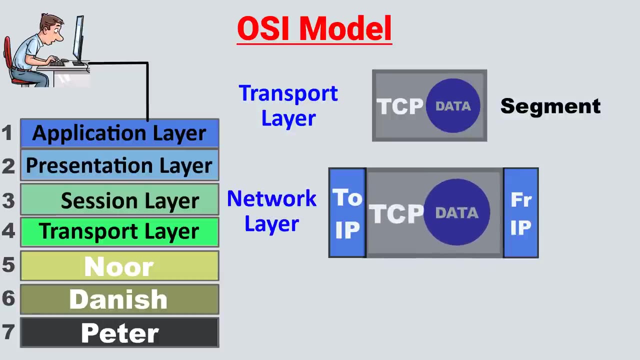 In that case we use UDP protocol. Normally voice and video streaming using UDP protocol to transmit data. So after that transport layer, send data segment to network layer. As per story, Tuba send segment to Noor and Noor put the to and from address on each segment. 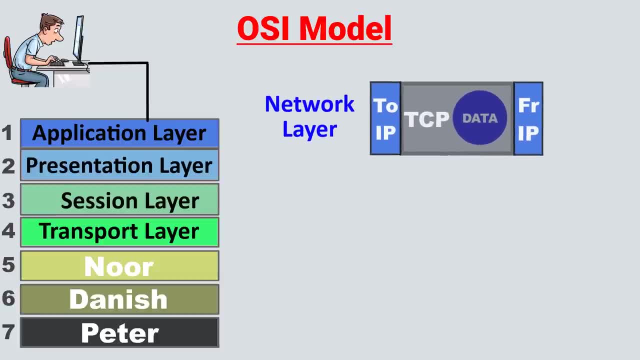 And decide the route. So the Noor mean network layer, as per the same model, And the function of network layer is logical, addressing routing and path determination of each data unit. Data unit in the network layer is called packet and this is the OSI layer where router exist. 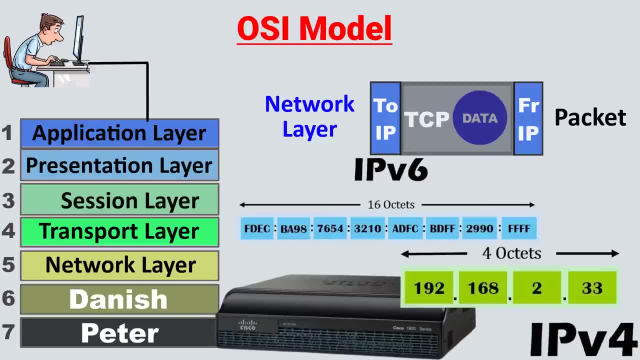 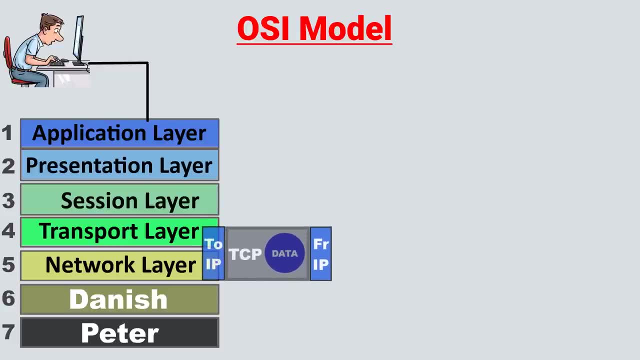 IPv4 and IPv6 addressing done on network layer and its called logical addressing. The network layer send data in form of network layer, Of packet to data link layer. So in the story Noor send packet to Danish. So Danish mean data link layer as per OSI model. 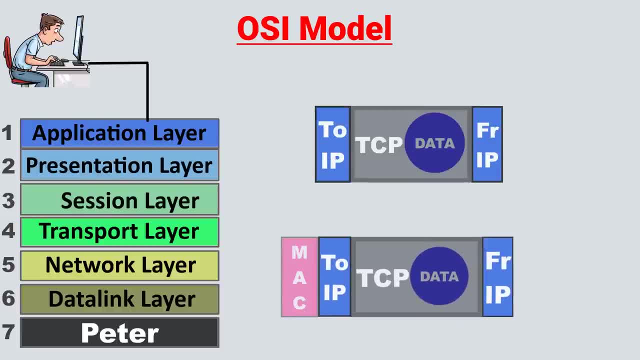 And in reality, what data link layer do He add sender and receiver MAC address on each packet? There are two type of addressing in network: Logical addressing and physical addressing. Logical addressing done on network layer, where sender and receiver IP address are assigned to each segment. 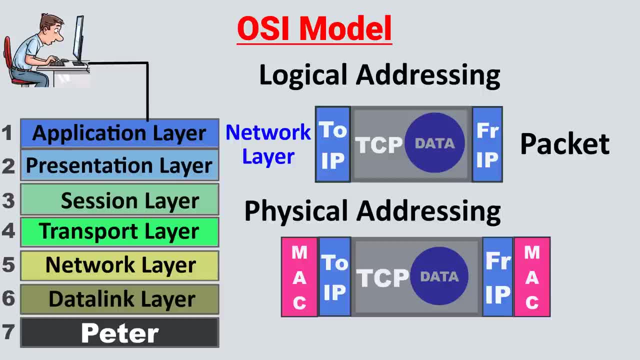 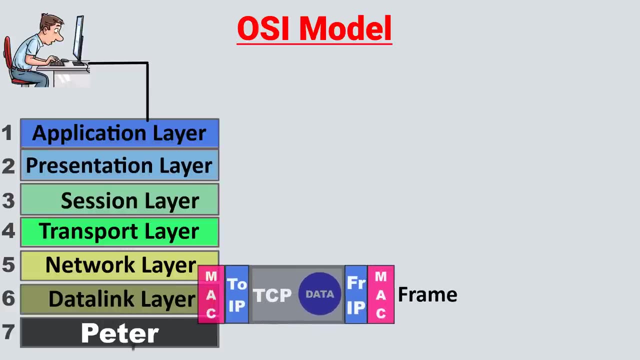 To find the IP address To form a data packet. It also called layer 3 addressing. Physical addressing are done on data link layer, where sender and receiver MAC address are assigned to each data packet to form a frame And then send this frame on physical media. 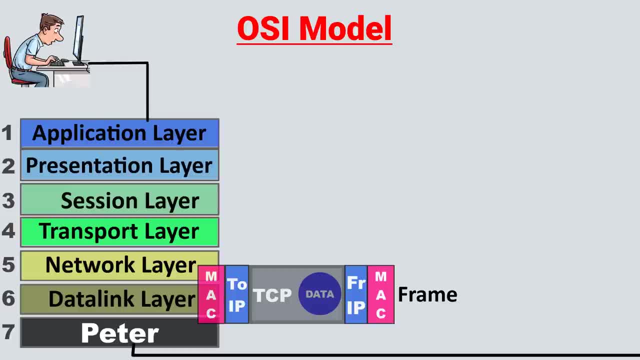 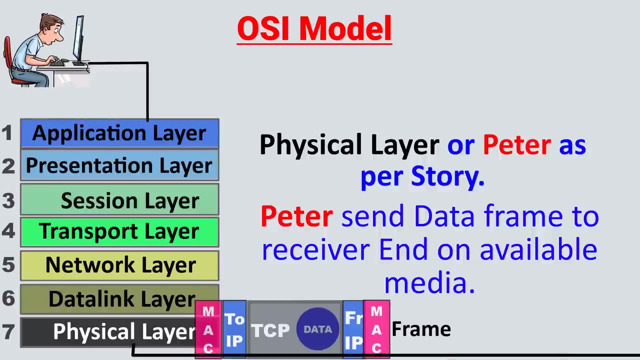 Like copper wire or optical fiber. Basically, data link layer allow upper layer of OSI model to access media using technique called framing. After that there is physical addressing, After that there is physical layer, or peter, as per story. What peter did in story, He just send data frame to receiver end on available media. 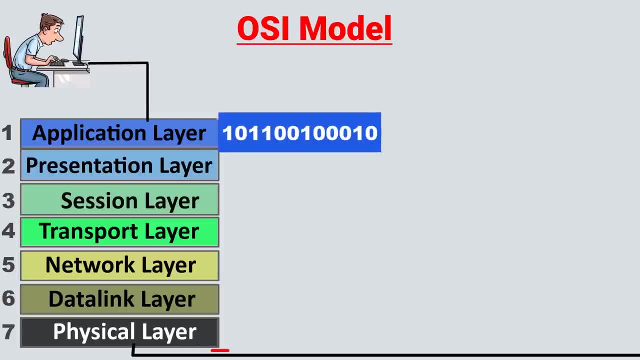 So in OSI model physical layer, convert this binary sequence into signals and transmitted it on local available media. It can be electrical signal in case of Ethernet LAN cable, or light signal in case of optical fiber cable. So the generated signal on physical layer depends on the signal. 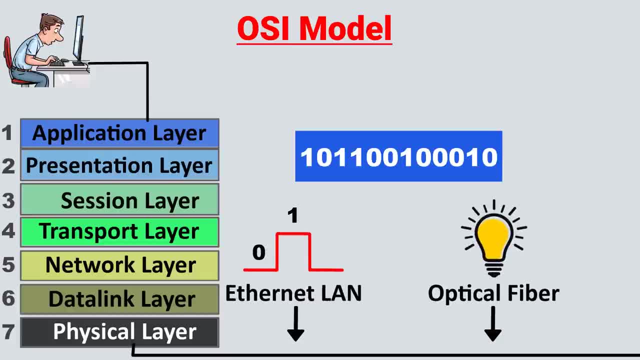 So the generated signal on physical layer depends on the signal. So the generated signal on physical layer depends on the signal. So the generated signal on physical layer depends on the type of media used to connect to devices. So that's it on sender side, as per OSI model. 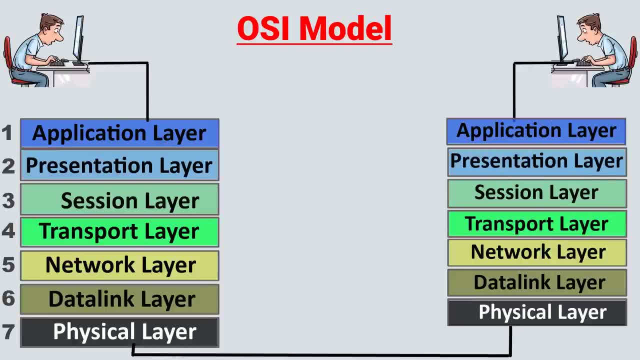 And when signal reach on receiver and physical layer, same process: what happened on sender side repeat on receiver side, but in reverse direction. Like when signal reach physical layer on receiver side in form of electrical or light signal, physical layer, convert them into binary bits 0 and 1.. 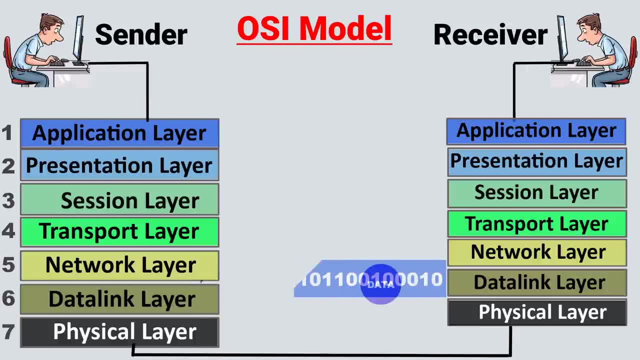 And send to data link: Data link layer. convert them into a frame and forward that frame to network layer. Network layer check to and from IP address and confirm this is his logical IP address and send these packets to transport layer. Transport layer: receive 4 packet and convert them into one segment and send that segment. 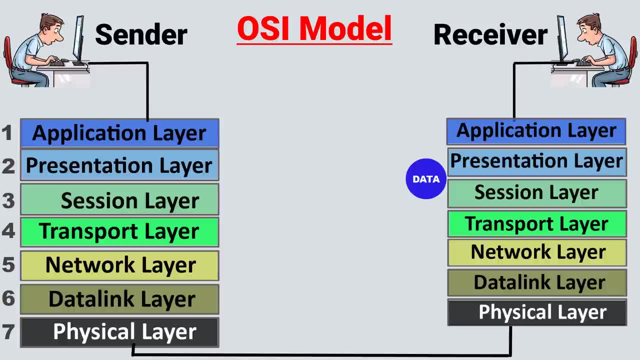 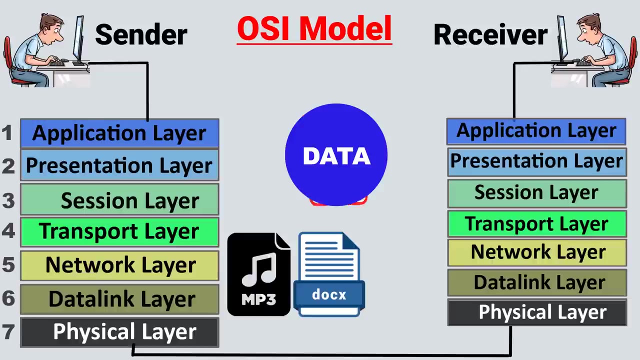 to session layer. After receiving on session layer. session layer send message to sender that they receive the data, or 400 pages as per story And session, or connection between sender and receiver disconnected, And session layer send this data to presentation layer. Presentation layer convert data into same format as it send, like mp3 or docx or pdf. 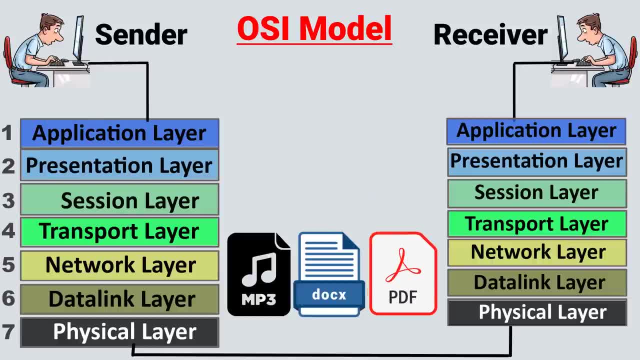 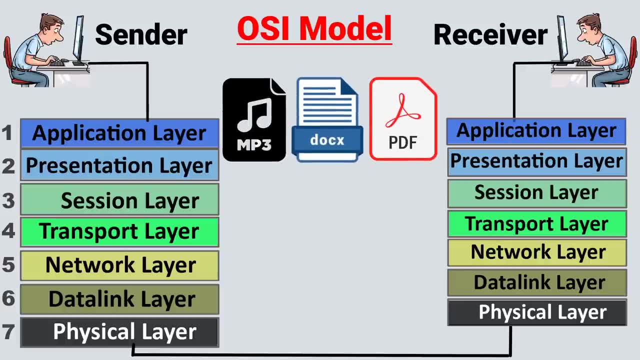 format So application can understand the data at application layer And application layer open that data on that specific application. So this is very simple and basic intro of osi model in form of OSI model. Thanks for watching of story Soon. I will make video for each layer of OSI model and will discuss more technically. 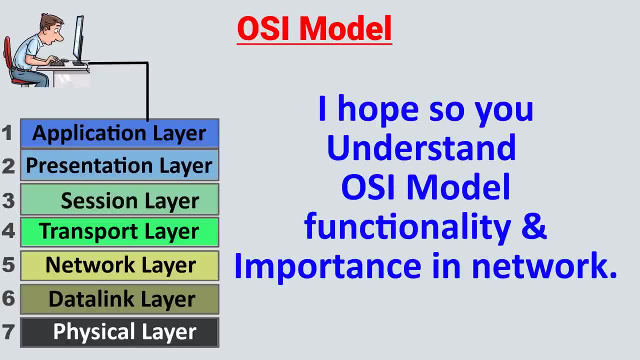 I hope so you understand OSI model functionality and importance in network. Thanks for watching my video and please don't forget to like and subscribe my channel.